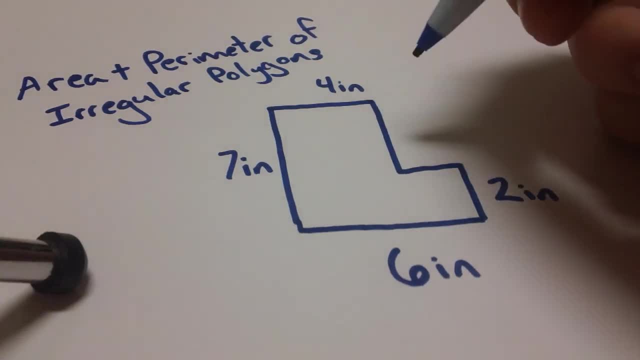 thinking outside the box. So what we want to do is we want to find the area and perimeter. We'll start with perimeter first, of course. That's almost always the easiest right, And perimeter is all of these sides added together. I always thought of it the way it was taught to me. 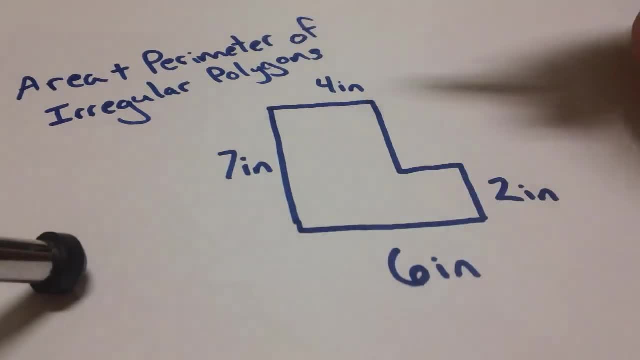 is kind of like if you had this shape and you were building a fence around it, right, How much fence would you need? Now we have four inches, seven inches, six inches, two inches, but unfortunately we have two sides here whose lengths are missing, right? So we got to figure those out. 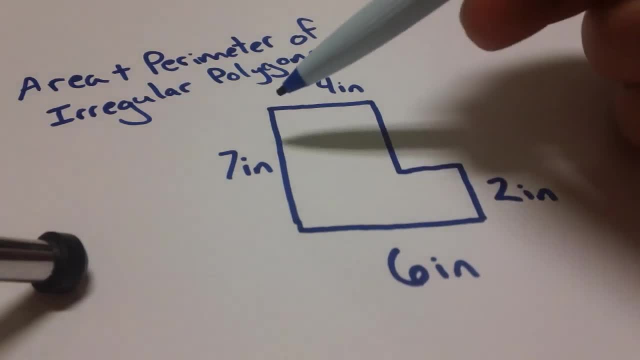 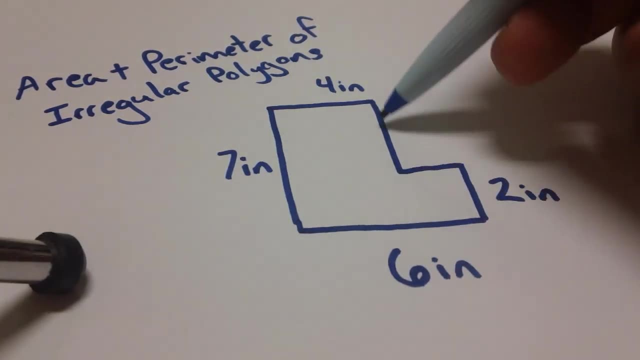 Now, this isn't too hard to figure out If you look at this and you just kind of think about it. this side here is equal to seven inches, This side over here is equal to two inches, And then we have this side here. 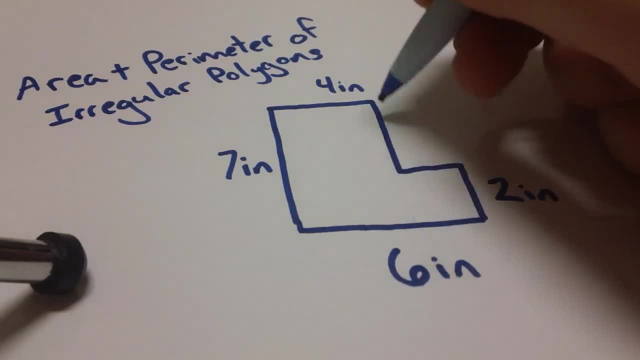 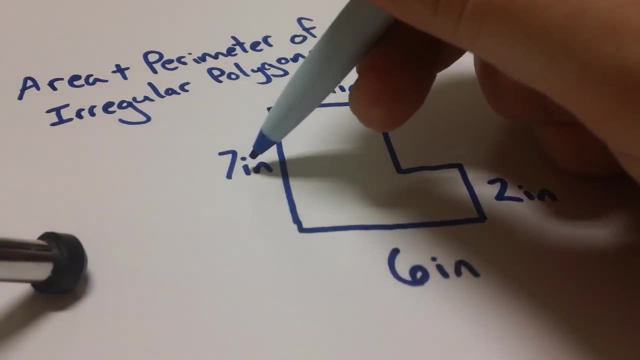 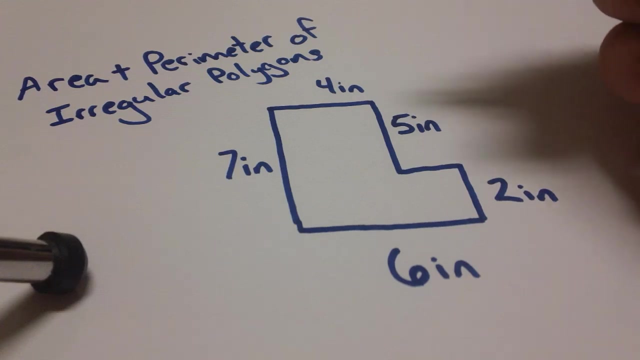 If you were to put these two sides together, they're going to add up to that seven inches, right? I mean straight up and down seven inches, So we can take that seven inches minus the two inches and get five inches. for this one It's just kind of like a missing part of a line segment. 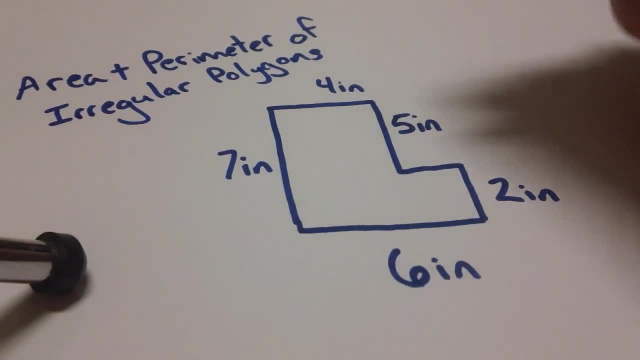 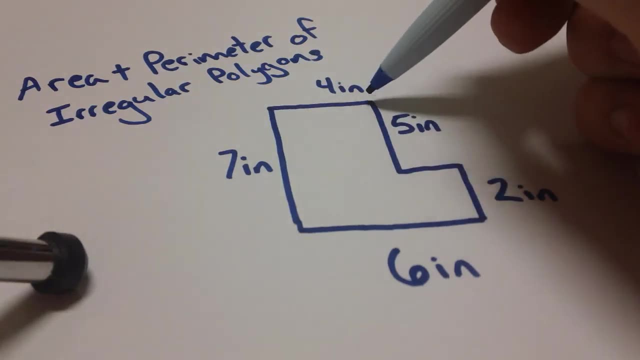 when you have two halves and you have the whole. Now for this one down here, we have six inches all the way across the bottom. Across the top, we have four inches here and then we're missing those two. but yet again, not too difficult. 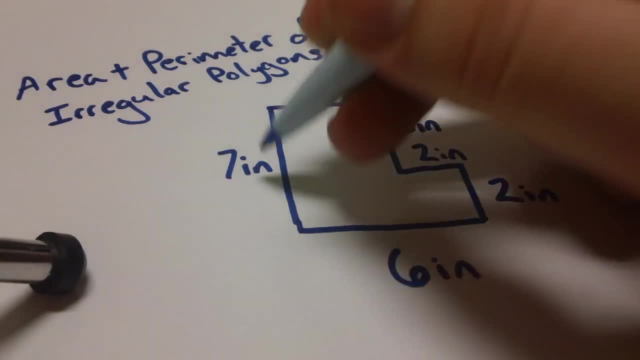 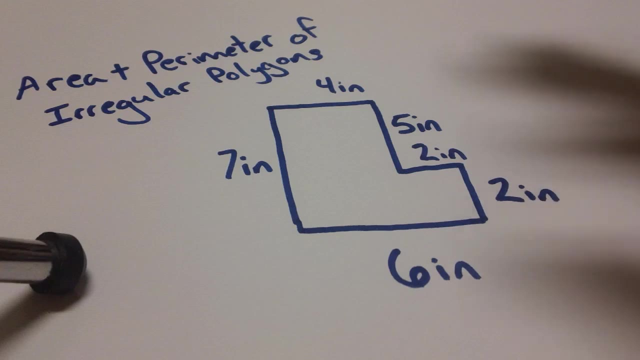 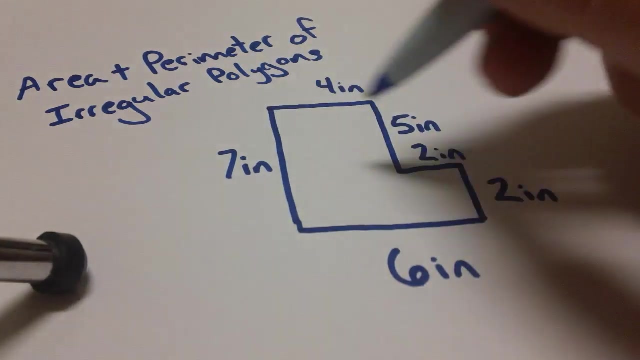 Six inches minus four inches, that's going to give us two inches, The sides opposite of each other. Whenever I have a shape like this, I always kind of like to think of it, just mentally, make it a square or a rectangle right, And just to understand that the sides opposite of each other. 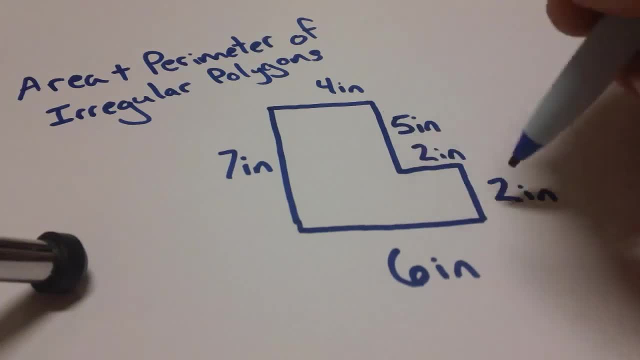 they're going to be equivalent, So we can use that information to help us find the missing ones. Anyway, perimeter seven plus four, we're going to get 11,, 11 plus five, 16,, 16 plus two, 18,, 20,. 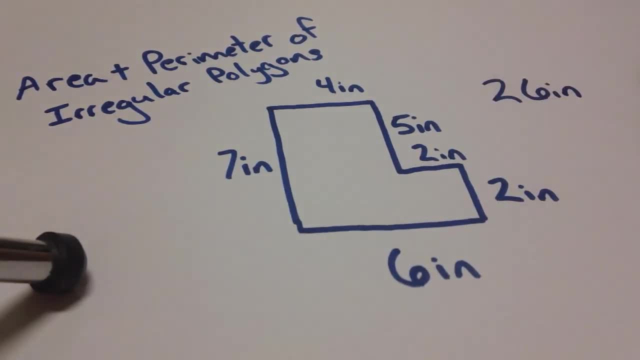 and then 26.. So our perimeter is in fact just going to be 26 inches. right, The area is a little different because, you know, there's not exactly an area formula for a weird looking shape like this. right, We don't have a formula for L shaped hexagons, but what we do have formulas for are rectangles and.